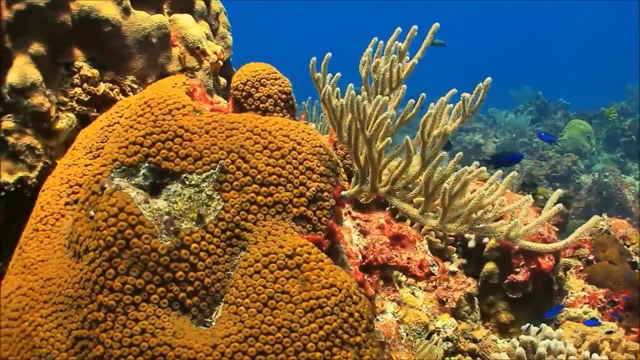 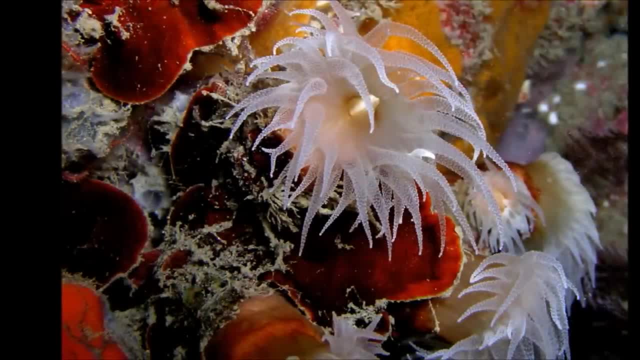 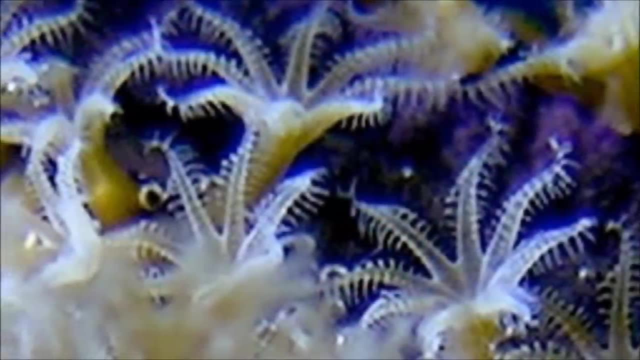 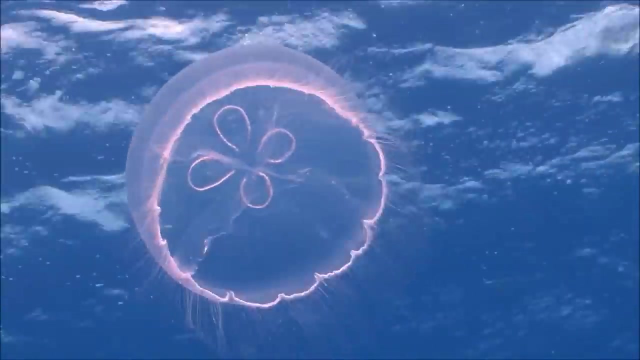 Coral reefs are only found in shallow tropical seas. They may look like colorful rocks or even plants, but coral is really an animal. Coral is built by polyps. Polyps are very small creatures that are related to jellyfish. Unlike the jellyfish, which propel themselves around through the water, coral are stationary. They grow together in a colony called a coral head. A small piece of coral may be made of hundreds of polyps, A bigger one may have thousands. Hard corals create the reef by secreting calcium carbonate or limestone, a type of rock which gradually builds up into a solid structure. Coral grows slowly, only a few. centimeters a year. It can take hundreds of years to form large pieces like this. Of course, not all coral is hard. Sometimes they can be very hard and sometimes they can be very hard. Coral types are soft. They may look like fans, bushes or feathers, but once again it is. 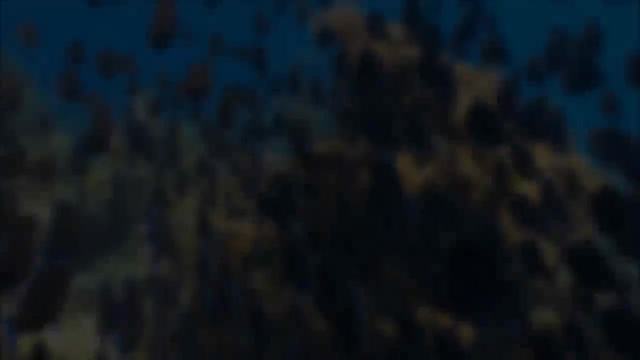 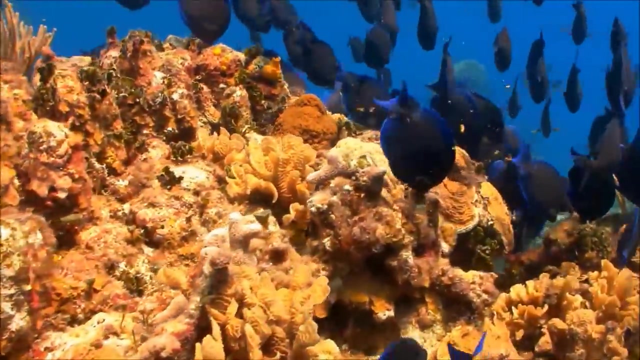 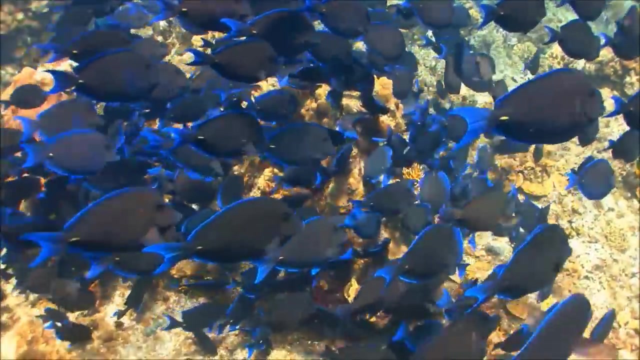 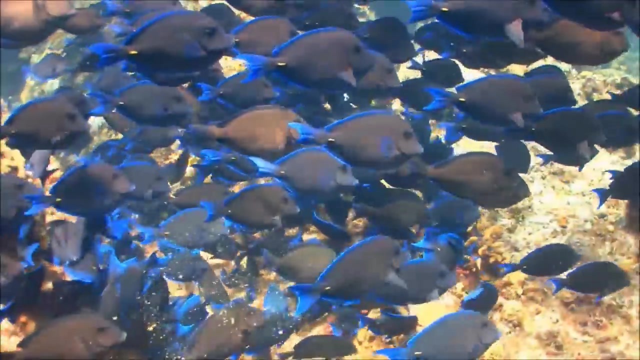 really a colony of tiny animals living together. When many corals grow close together, it's called a reef. Reefs provide very important habitat for fish and other sea creatures. Coral provides shelter for little fish- a place to hide. Not many small fish in one place attracts big fish, which in turn attracts big predators. 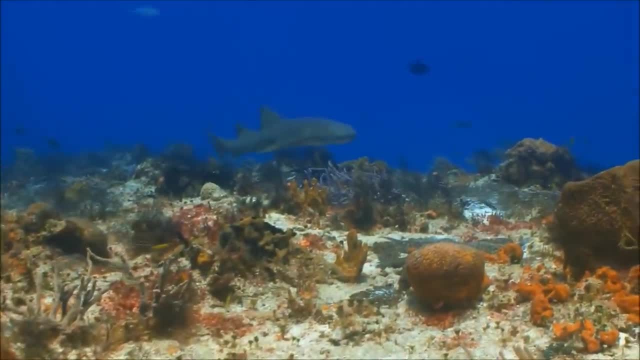 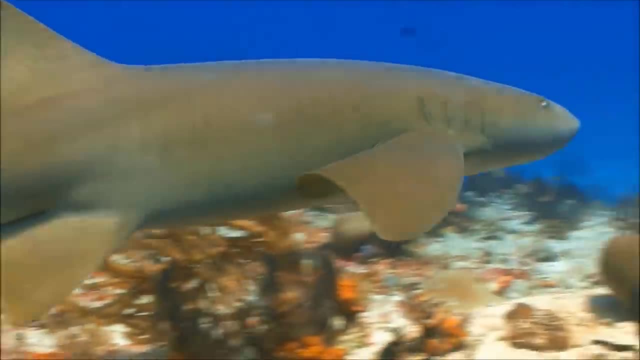 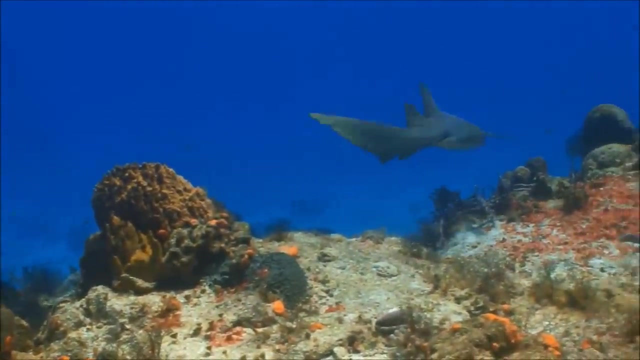 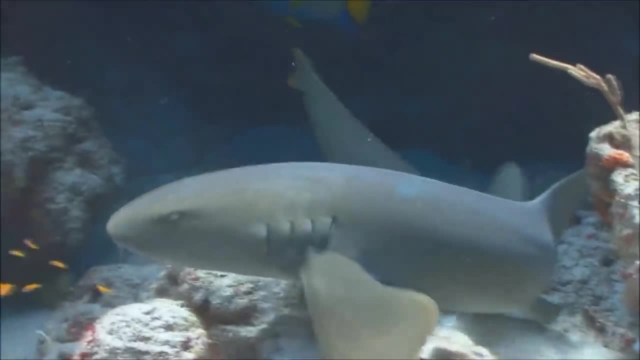 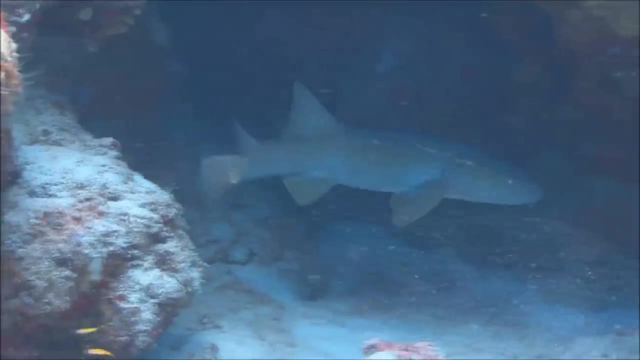 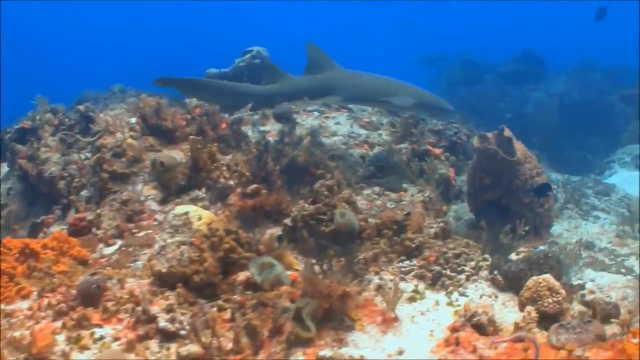 Nurse Sharks are slow moving bottom-dwellers and, for the most part, harmless to humans, although they can grow up to 14 feet in length. Their strong jaws allow them to crush shellfish and even coral if need be, but they prefer. 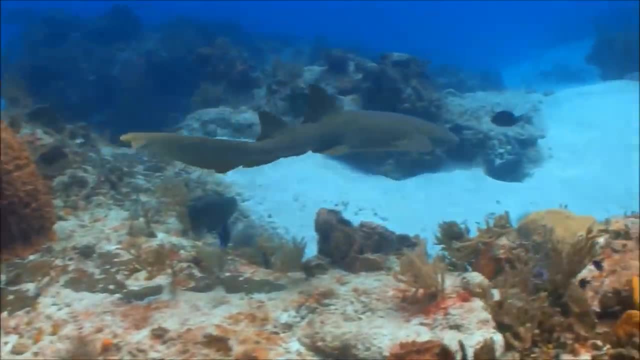 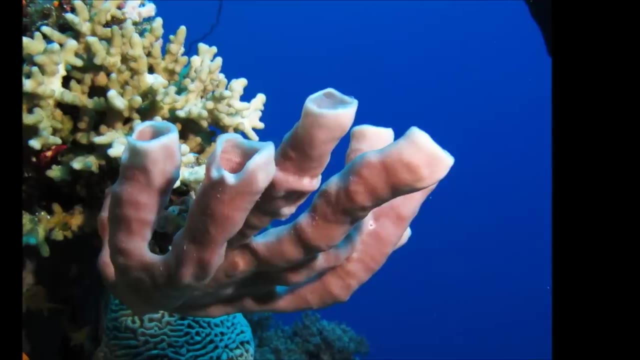 to eat shrimp, fish and squid. The reef also provides a place for algae. When coral seep into reef shells, they usually squint their ears, gulp them down. what with and sponges to grow. This provides food for a variety of creatures, for example the sea. 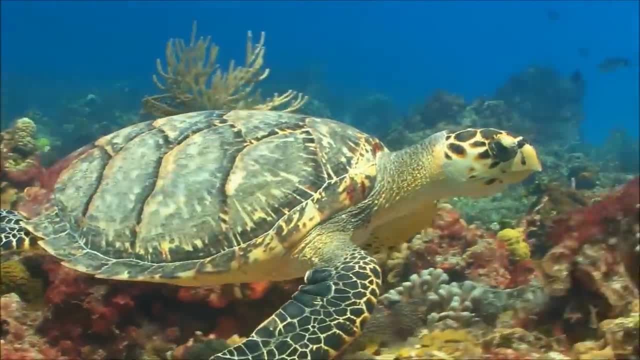 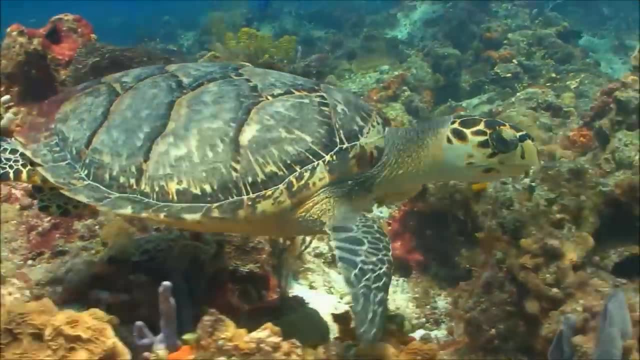 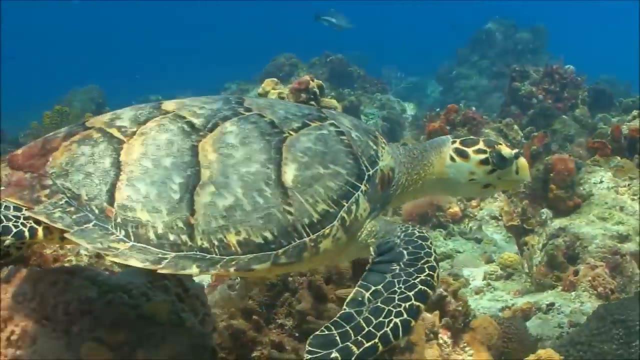 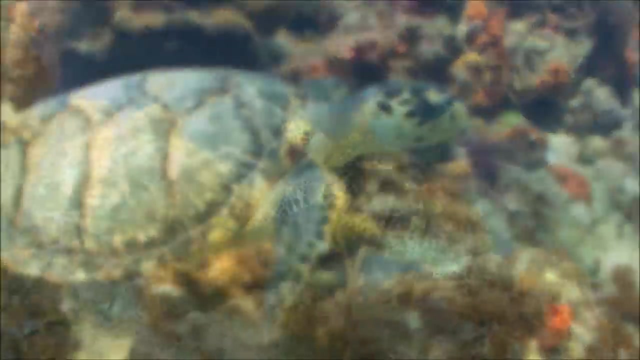 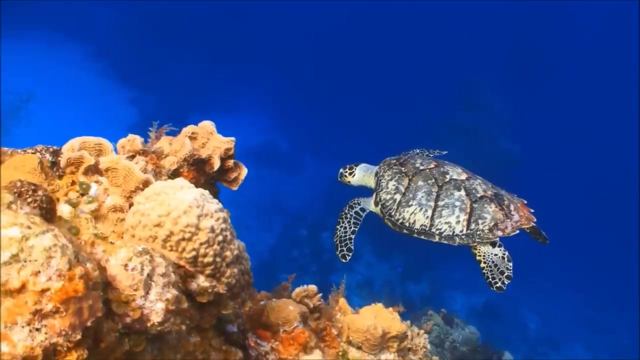 turtle. The hawk spill sea turtle, like most other kinds of sea turtles, is endangered, Hunted for their meat and for their shells, trapped in commercial fishing nets to drown and sickened by pollution. their populations are declining. These turtles rely on the food that grows on the coral reef and the reef in turn. relies on the turtles. It's a partnership that benefits both creatures. The turtles get a reliable source of food. The reef system gets a level of food. It's a less obvious advantage Without the turtles coming to eat the algae and sponges. they would overgrow the reef. 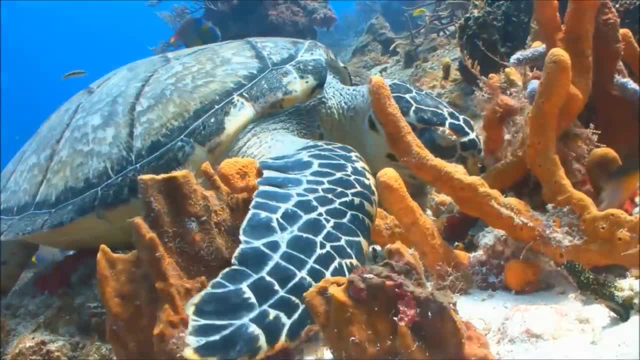 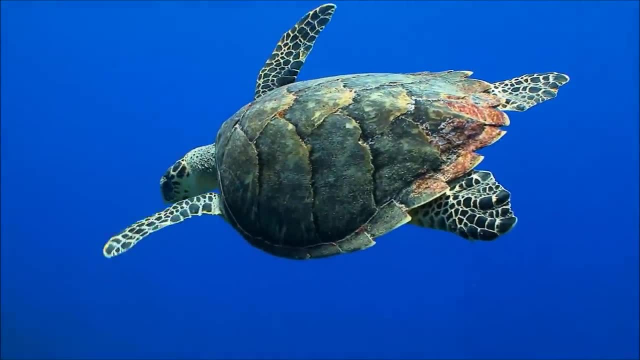 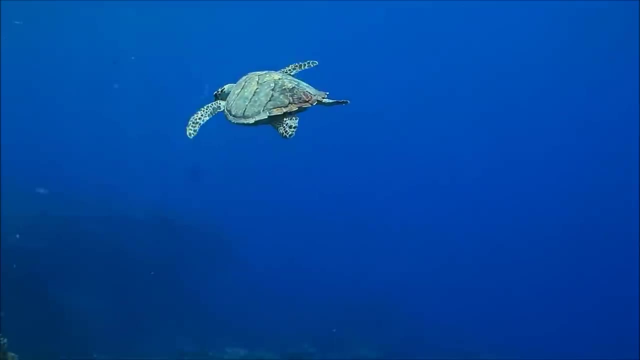 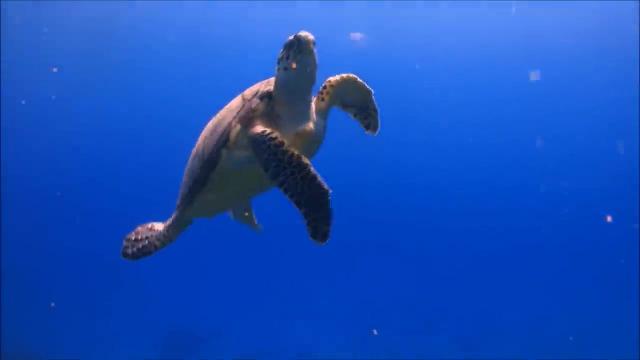 preventing the coral from growing and expanding. With lowered turtle populations in oceans worldwide, the health of coral reef systems will suffer. It is important for people to do our best to protect these peaceful reptiles, not just for their sakes, but for the health of the. 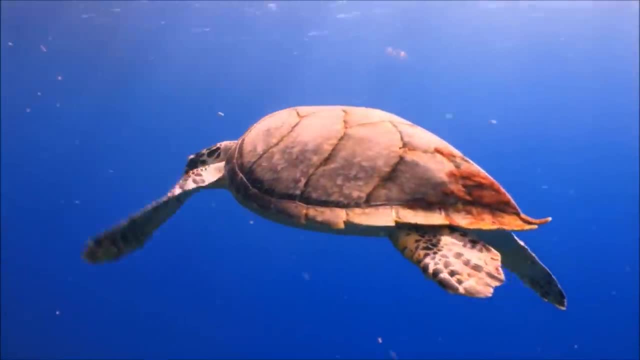 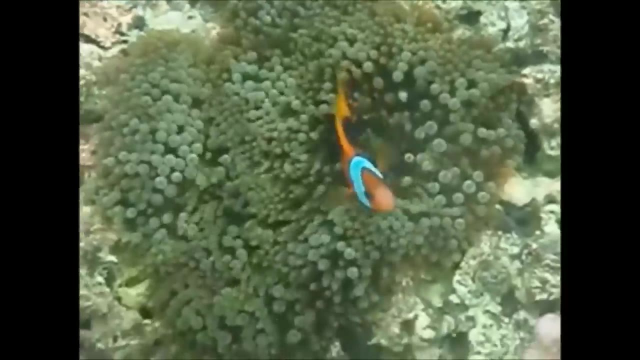 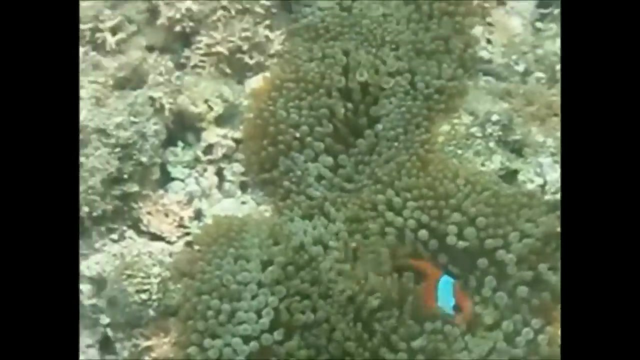 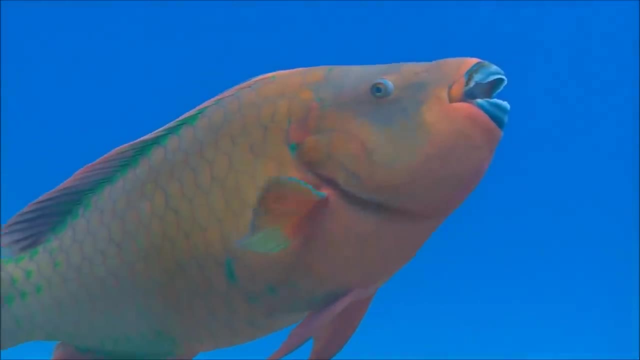 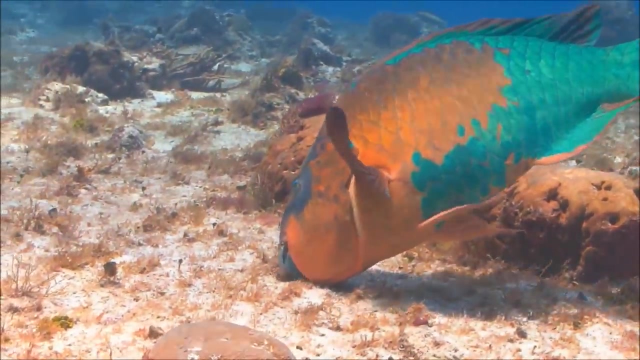 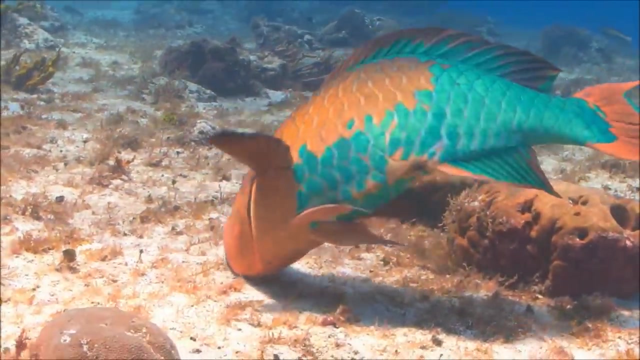 we're going to talk about today. Can you guess what parrotfish and beeches have to do with each other? Parrotfish are a distinctive family of fish species with a tough, bony beak so strong that they can bite through rock and coral. They do this so that they can eat the coral. 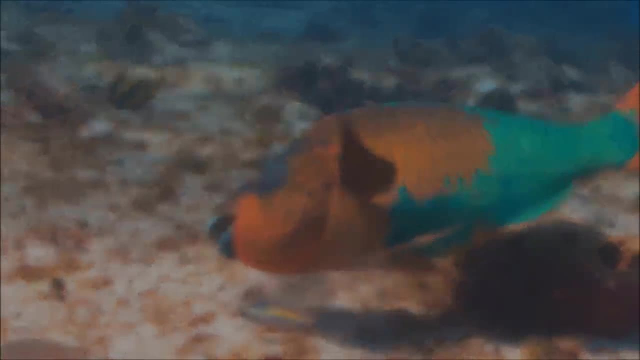 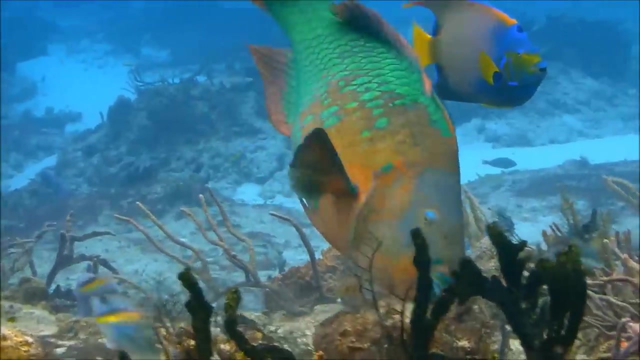 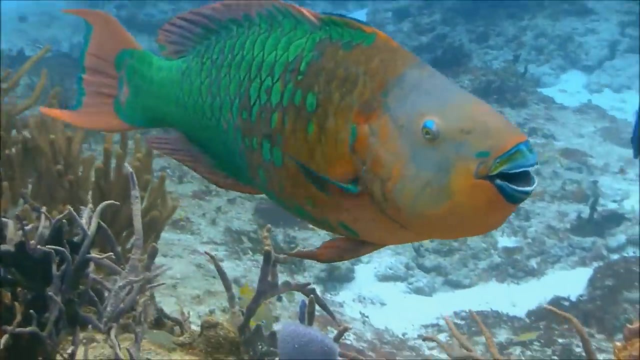 polyps and algae inside The coral is ground up and all of the edible parts are digested until only the limestone remains. Then the parrotfish has to get rid of all the crushed limestone, and there's only one way to do that: The parrotfish will excrete or poop. 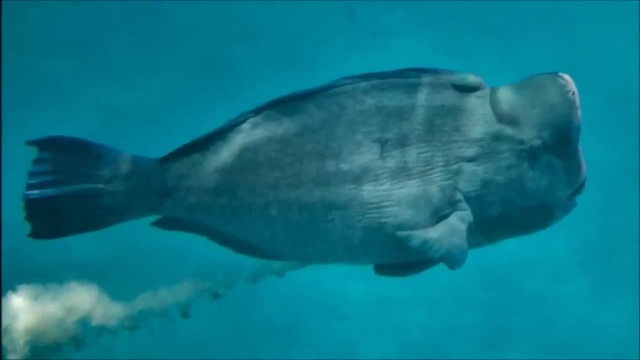 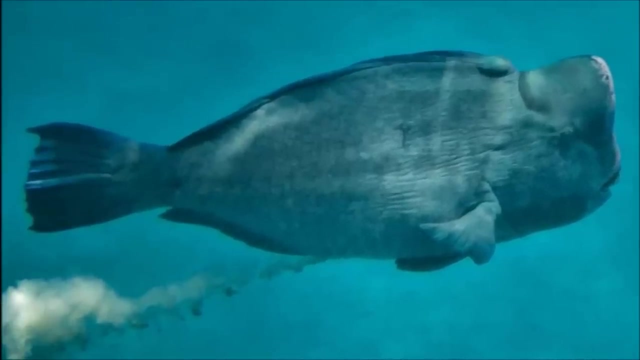 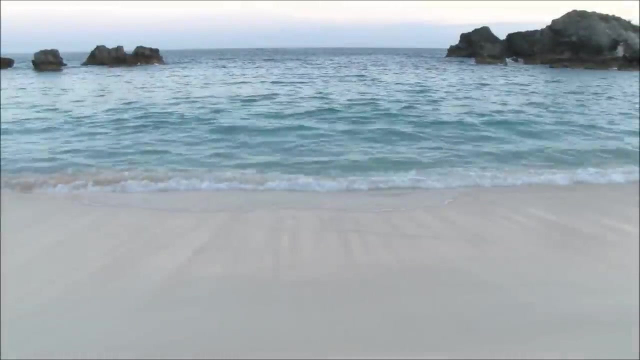 out the limestone, which has been crushed into a fine sand. In this way, a single parrotfish can produce 200 pounds or 90 kilos of sand every year. You heard that right. The next time you bury your toes in soft white sand at the beach. 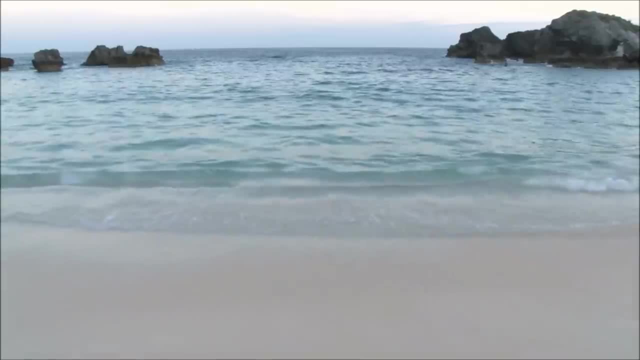 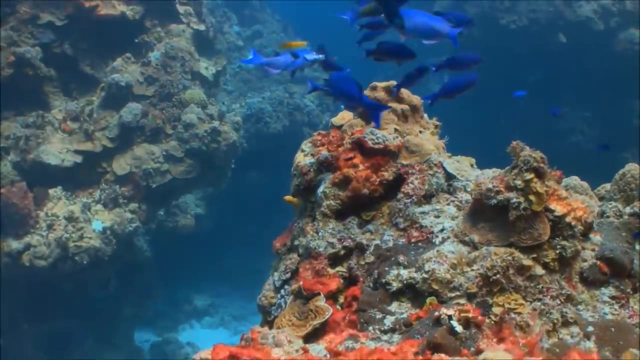 just remember you're making castles with fish poop. Coral reefs are sometimes called the rainforests of the sea. Coral reefs are sometimes called the rainforests of the sea. Coral reefs are sometimes called the rainforests of the sea. 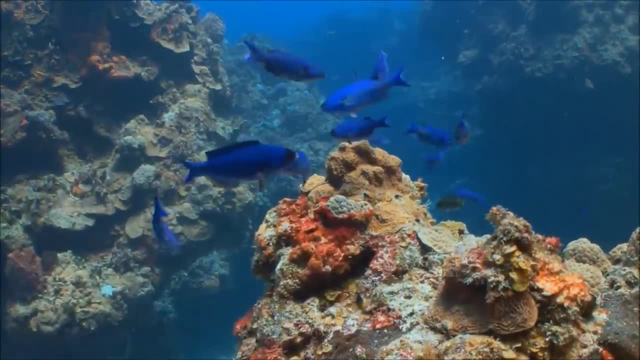 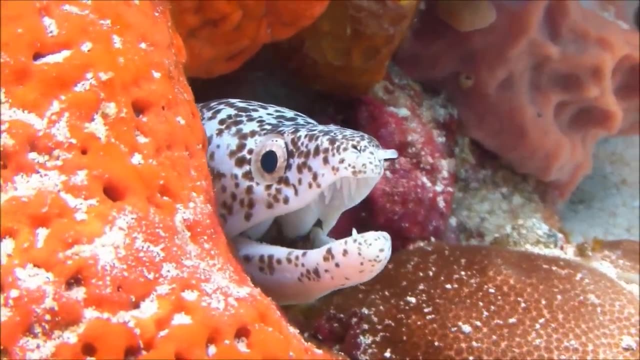 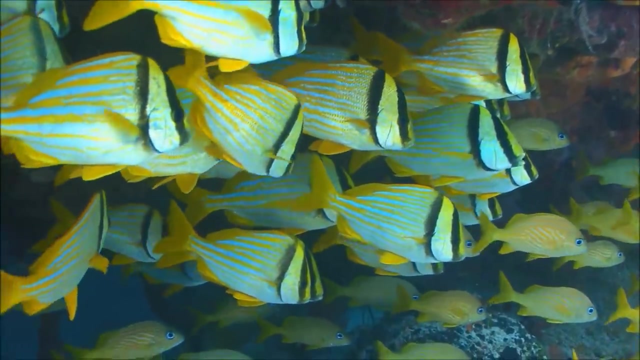 Though they cover only a tiny area of the ocean, they provide a habitat for a quarter of ocean animals. Unfortunately, the coral reef ecosystem is a fragile one. The delicate balance between the coral algae, fish and animals that live there is easily disrupted. 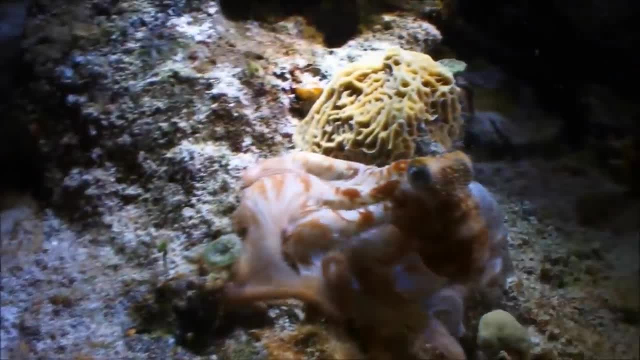 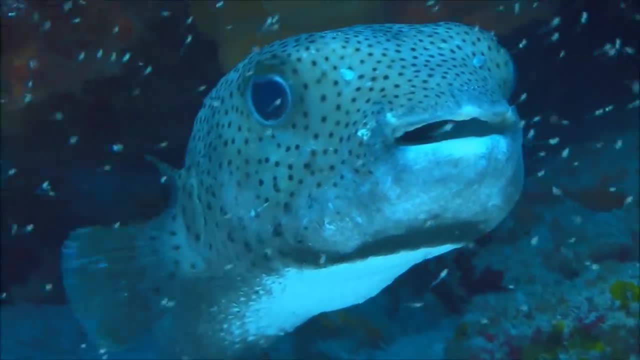 Overfishing by humans, ocean pollution and warming temperatures have all been caused by coral reefs. Most coral reefs are not protected by the World's most advanced ocean environments, The world's most advanced ocean environments, such as the Atlantic, the Atlantic, the Arctic. and the Pacific are all put the world's coral reefs at risk. Right now, more than half of the world's reef systems are in danger of destruction, and if nothing changes, then within 15 years nearly all the coral in the world will be. 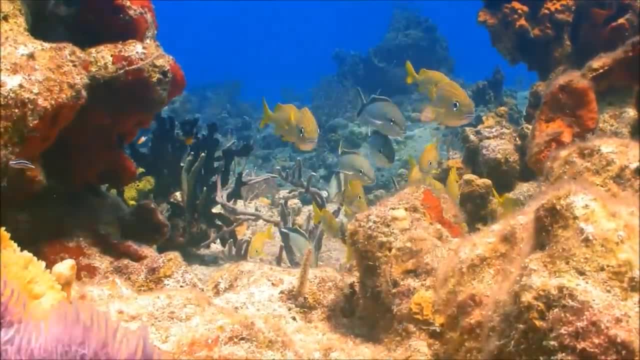 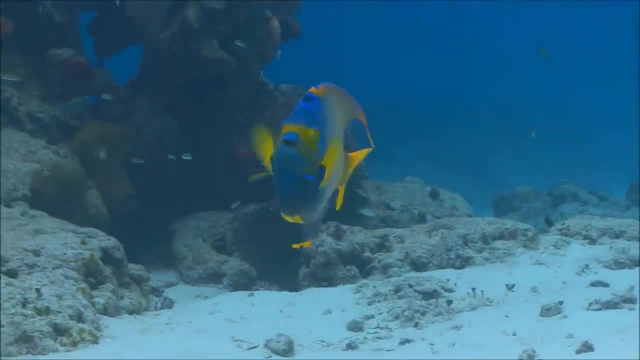 in danger of dying and disappearing. Fortunately, there are some simple things you can do to help protect coral reefs. Be careful not to waste water or pour chemicals down your reefs. Coral reefs are often the most dangerous and dangerous species of life. Coral reefs are often the most dangerous species of life. 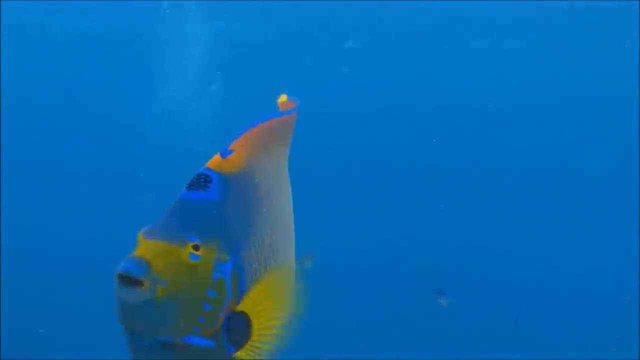 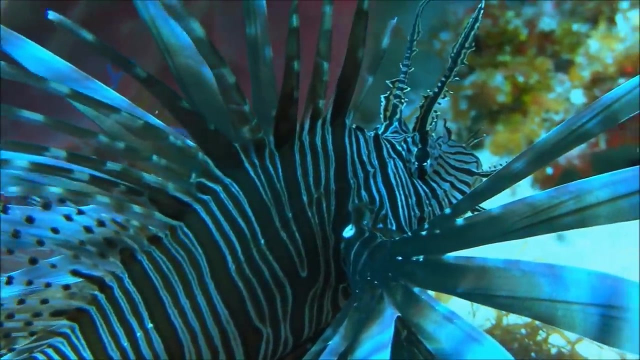 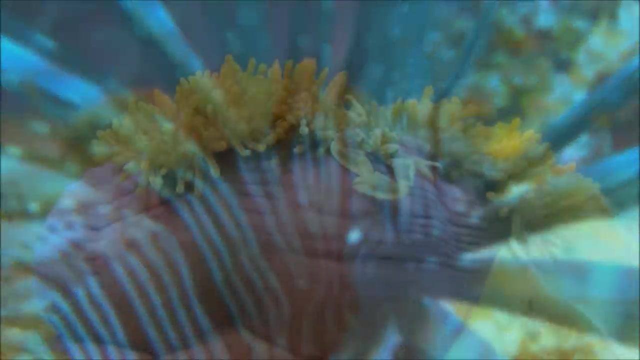 drain, since eventually, the water you use will reach the ocean and can increase pollution. Pick up trash that you see on the ground and recycle what you can so that garbage won't find its way into the water. Most importantly, make sure people know that you want to protect the coral reefs, so that 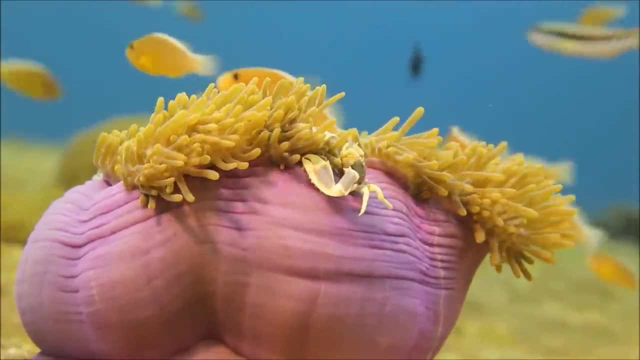 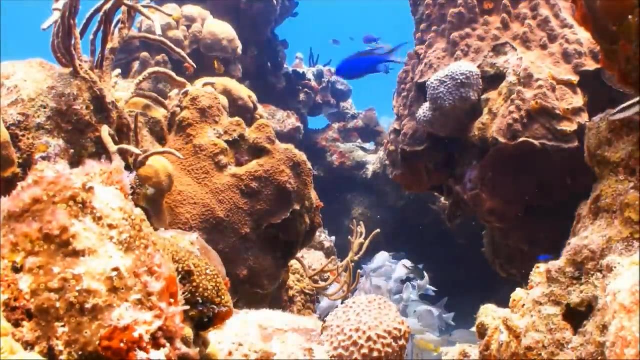 when we make decisions about how to take care of our world, we will make choices that will protect the reefs. I hope you learned something new exploring the reef with me today. Goodbye, till next time.